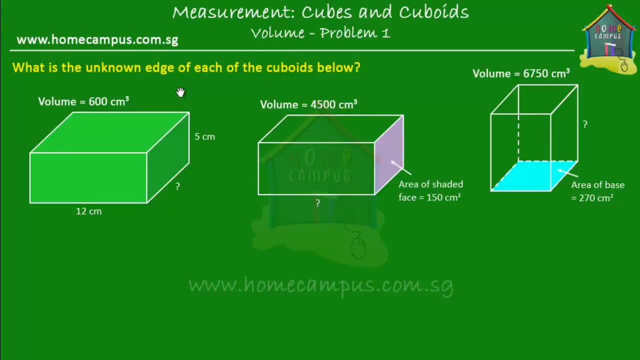 Hello and welcome to homecampuscomsg. In grade 5, we learned that the volume of an object is the space occupied by that object. Okay, in terms of cuboids, how we measure that space or the volume, is by finding out the product of its three edges. 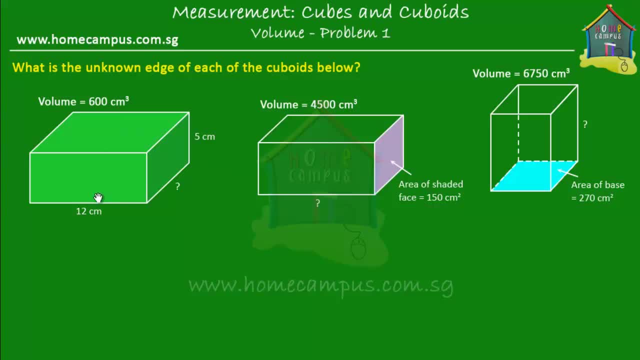 So in the case of cuboid- like, for example, this cuboid over here, the green one- the volume of this cuboid will be equal to the product of its length, its breadth and its height. Alright, now, what we'll do in this lesson is solve a few questions based on the knowledge that we gained in the smaller classes. 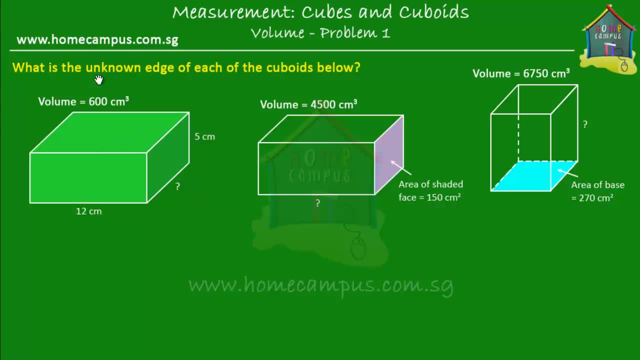 Alright, so let's start by reading out the question first. It says: what is the unknown edge of each of the cuboids below? So we've got three cuboids here: a green one, a pink one and a blue one. okay, 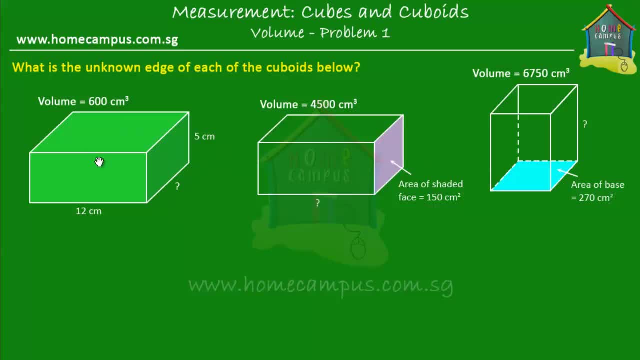 And we have to find out the edges that are unknown. In the first figure here, this side is unknown. In the second figure, here, the longest edge is unknown. And in the third figure, here, the height is unknown. okay, So let's solve these questions one by one. 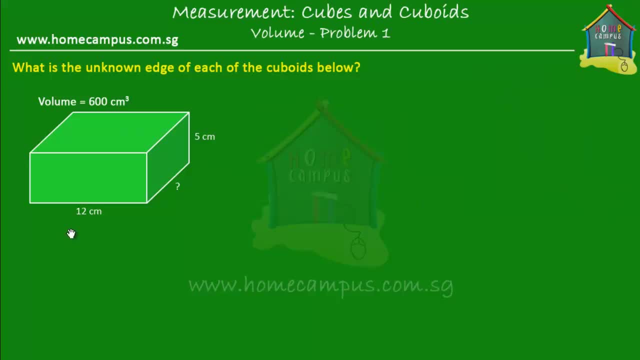 So let me hide the other two figures and let's concentrate on this figure first. okay, So the volume of this cuboid over here is given to us, It's 600 centimeter cube. okay, Now, this seems to be the longest side. 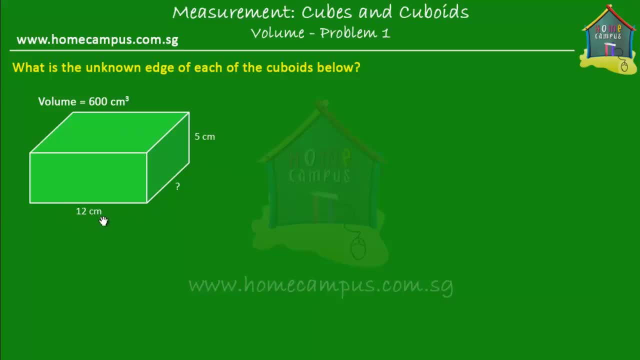 So this is the length. The length is given to us. It's equal to 12 centimeters. The height is given to us, Which is 5 centimeters. Now, the breadth or the width is unknown. Now, we said just now that the volume of a cuboid is the product of its length, its breadth and its height. 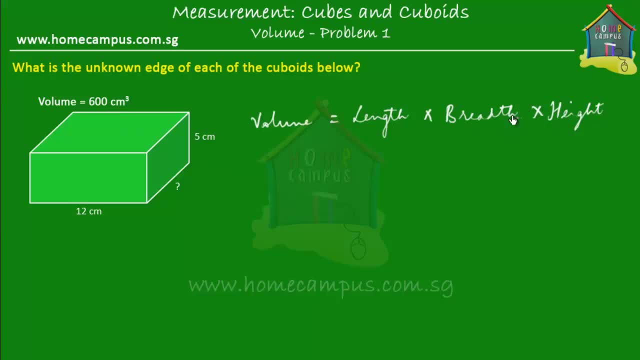 So volume is equal to length times breadth, times height. Now, from the numbers that we know here- the volume, the length and the height- can we find out the breadth? Yes, we can very easily. Well, how so? 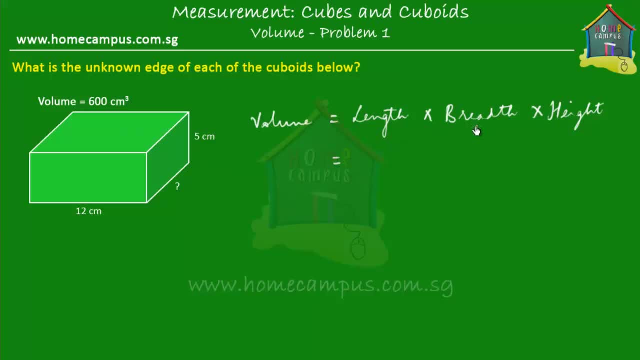 Let's see. okay, So volume is equal to length times breadth times height. If we do a bit of shuffling here, it's equal to length times height times breadth. All I did here was move the breadth to this side and the height to this side. 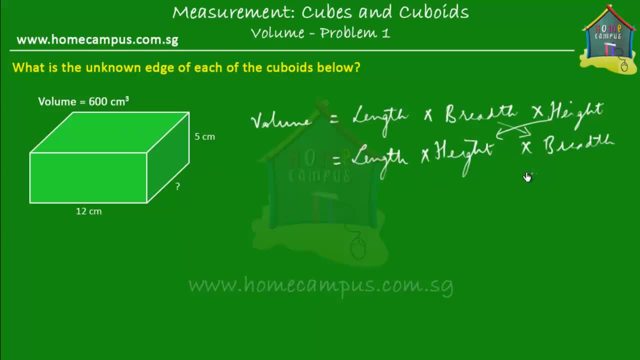 And since these are all products, all just multiplies, so this doesn't change the answer. So, okay, now, if you want to find out the breadth from here, how do we do that? Well, we have volume, okay, So we know the volume. 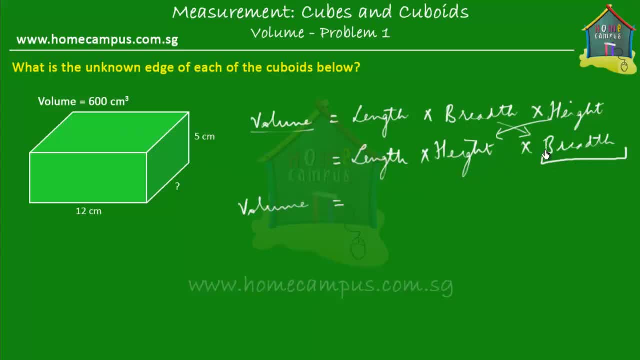 Volume is equal to length times height times breadth. But if you want to find out the breadth, okay, then what do we do with this part over here? the length times height? Well, we simply divide that by volume. We move it to the other side of the equal sign. 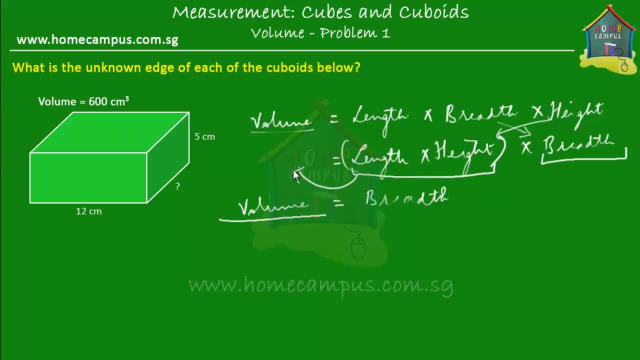 So if we move this to the other side of the equal sign, then this becomes divided by: okay, So the volume is divided by the length and the height. to give you the breadth. So breadth is equal to volume over length times height. Very simple. 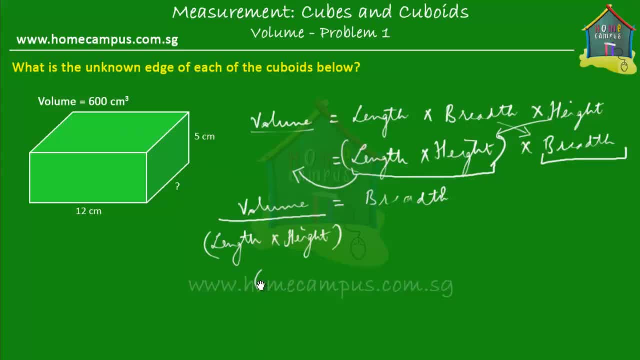 Now we know the numbers for volume. It's equal to 600 centimeter cubed, so we put 600 here. We know the numbers for length and the height. Length is equal to 12. And height is equal, So this is 600 over 12 times 5.. 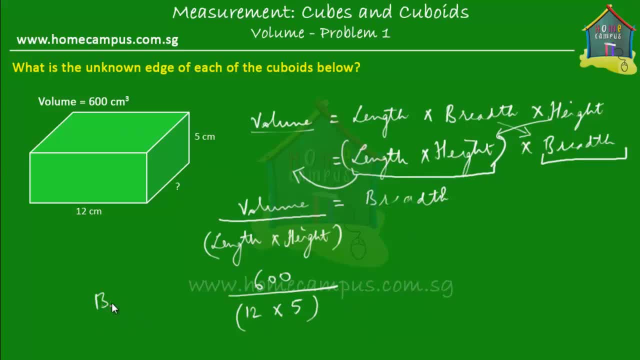 That's what your breadth is equal to. okay, So breadth, I'll write that down here So we have room to do our calculations. Okay, so breadth is equal to 600 over 12 times 5.. Now, what is 12 times 5?? 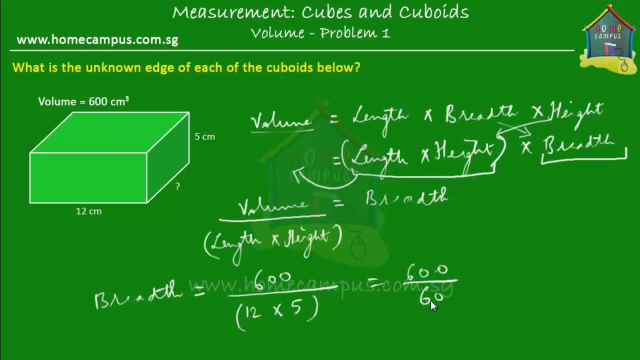 Well, 12 times 5 is 60. So it's simply equal to 600 over 60, or 600 divided by 60. Now how do you simplify that? Quite easy: The 0 and the 0 cancel out 60 divided by 60.. 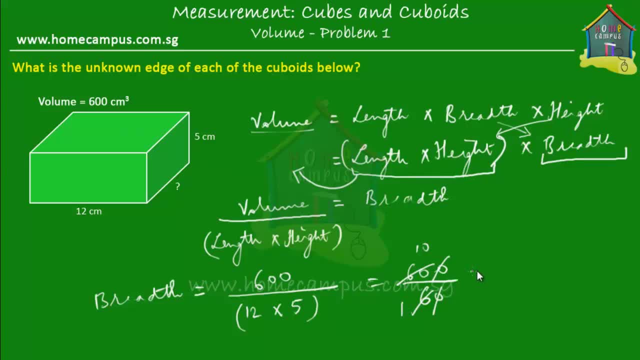 6 gives you 10.. 6 divided by 6 gives you 1.. So this is simply 10 over 1, or just 10.. So as simple as that. your breadth is equal to 10 centimeters, So this breadth over here is equal to 10 centimeters. 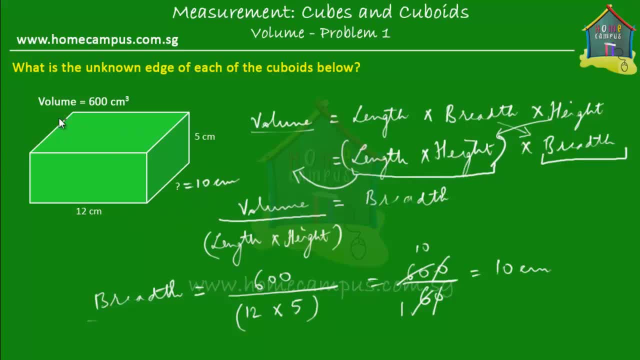 That's it. Now, just to double check that we got the answer correct, let's find out the volume using the length, the breadth and the height. okay, So length is 12 times breadth is 10 times, height is 5.. 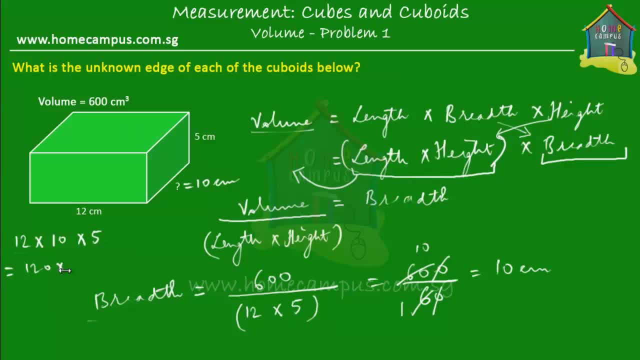 Okay, 12 times 10 is 120 times 5.. Okay, 120 times 5.. Well, let's do that 120 times 5.. How much is that? 5 times 0 is 0.. 5 times 2 is 10.. 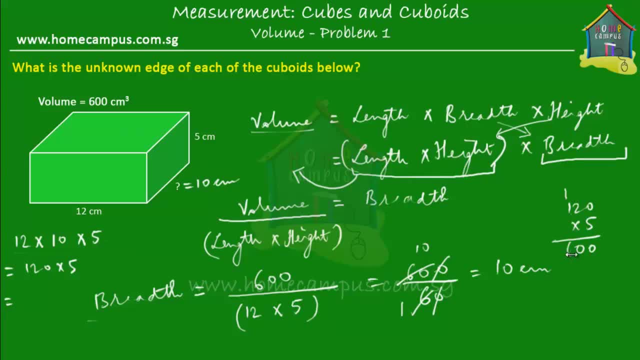 And 5 times 1 is 5, plus the 1 carried over, which is 6.. So, yes, 120 times 5 is equal to 600.. And that is your volume, which was given to you: 600 centimeter cubed. 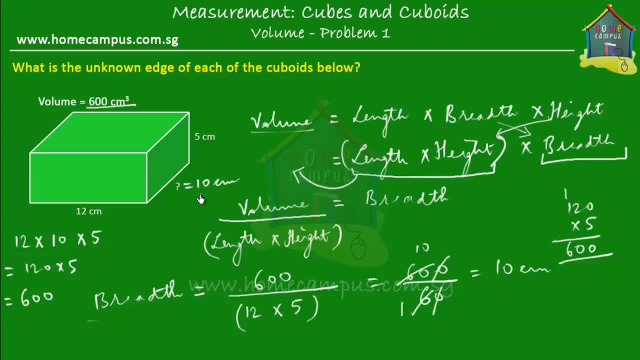 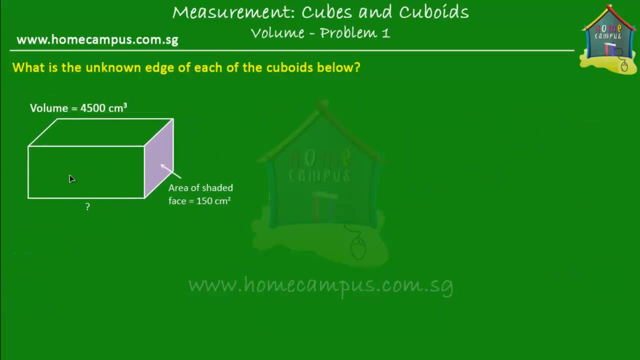 So the unknown edge in this figure is the breadth, which is equal to 10 centimeters. All right, shall we move on to the next one now? Okay, here is your next figure. Let me move it to the side. In the next figure, what's given to us is the volume, which is 4,500 centimeter cubed. 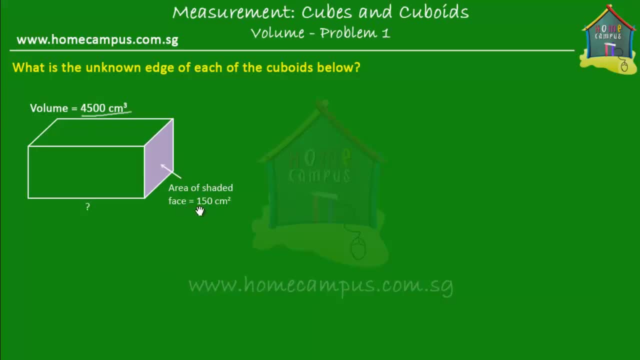 And the other thing that's given to us is the area of the shaded face, which is 150 centimeter squared, And what we have to find out is the length. All right, Now we put down the formula again: Volume of a cuboid is its length, times its breadth, times its height. 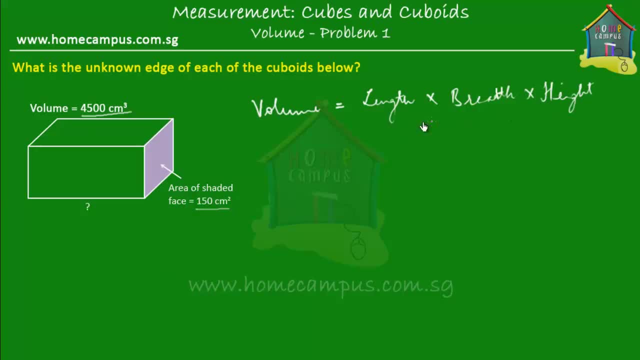 So volume is equal to length times breadth, times height. Now how do we find out what the length is equal to, given whatever information that we are given? Let's see. Do we know what the breadth is equal to? No, we don't know what the breadth is equal to. 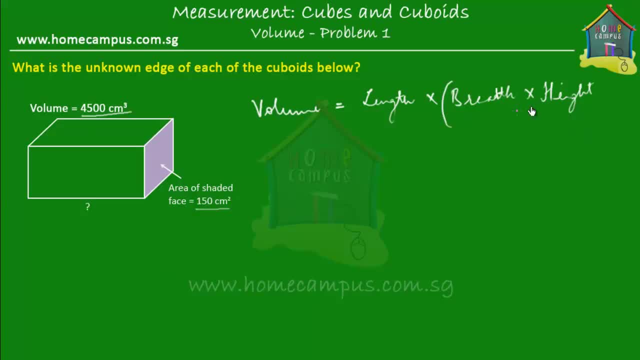 Do we know the height? No, we don't know. No, we don't know what the height is equal to. But we do know what the product of the breadth and the height is, Because we know what the area of the shaded face, the face that is made of the breadth and the height, is. 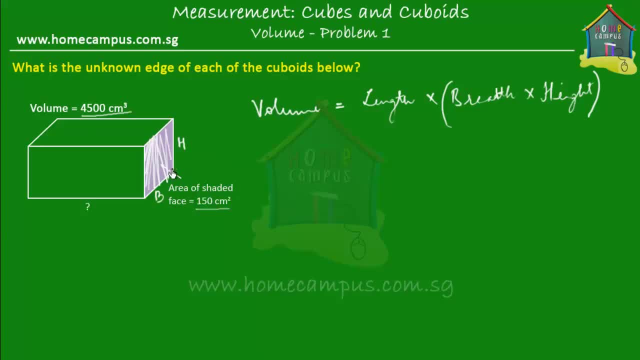 Well, this face over here is made of the breadth and the height. right, This is the breadth of the cuboid, this over here, and this is the height of the cuboid. Now, this face is a rectangle And its sides are equal to the breadth and the height of the cuboid. 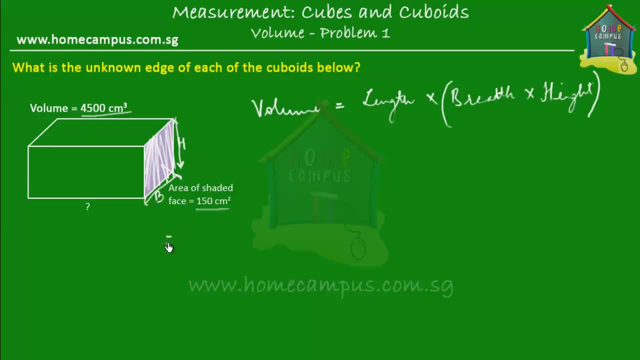 So in short, the area of the rectangle is equal to the breadth times the height, Or the product of the breadth and the height, which is over here right. So into this formula we can fit the product of the breadth and the height as the area of the shaded face. 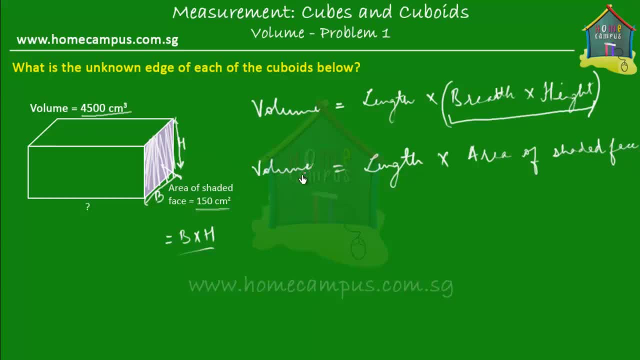 So in the case of this cuboid, the volume is equal to length times the area of the shaded face. Now can we find out what the length is equal to from this formula? Quite easy: Length is equal to volume divided by the area of the shaded face. 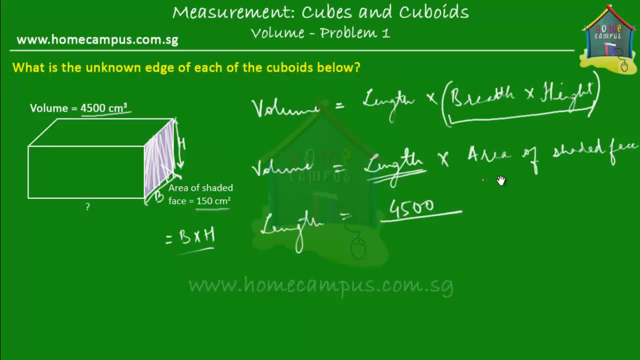 Now volume is equal to 4500 centimeter cube And the shaded face has an area of 150 centimeter square. Now We simplify this to get our answer: 15 times 1 is 15.. 15 times 3 is 45.. 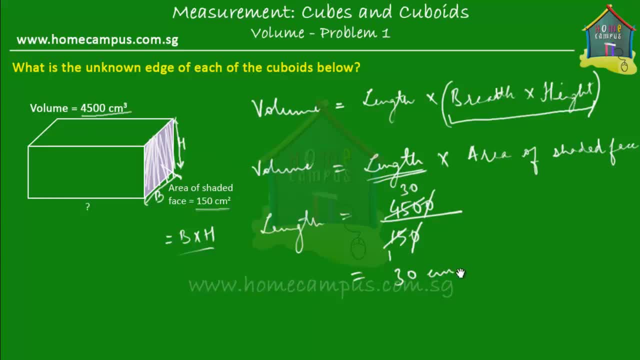 So you get 30 over here. So the length is equal to 30 centimeter. square, That simple. So your unknown edge over here is equal to 30 centimeters. If you want to double check, all you have to do is find the product of 30 and 150 and you should get 4500, which is the volume. 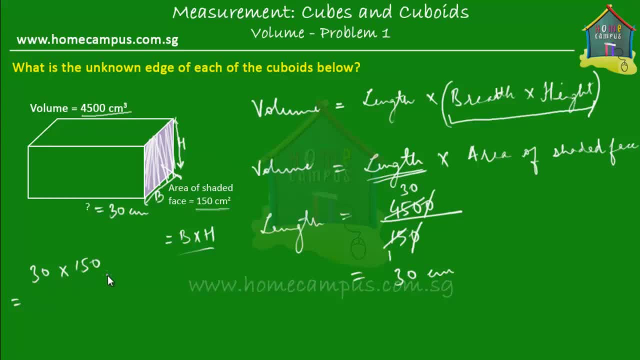 Okay. So you multiply the length and the product of the breadth and the height and you should get 4500.. Let's see if we get that. Well, 3 times 15 is 45. Okay, And the two zeros? 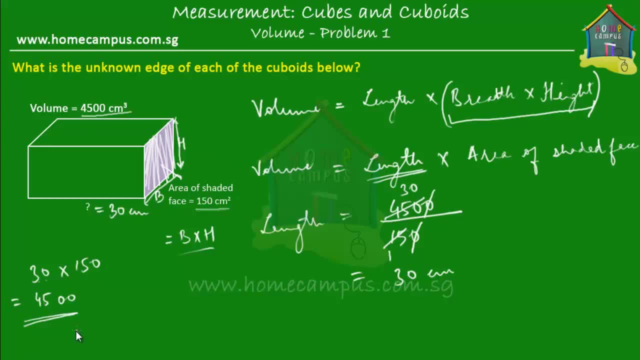 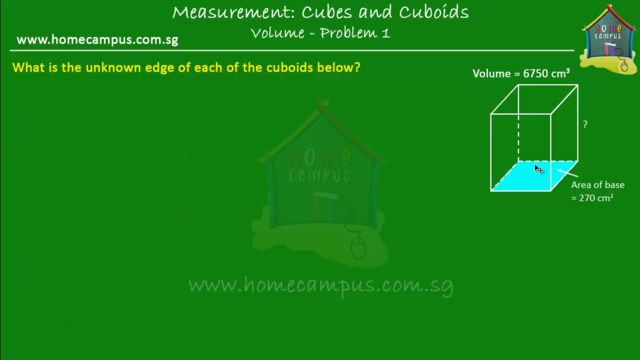 So we put that here And yeah, that is equal to 4500.. So that's it about this part of the question. Let's move on to the last figure. So this is your last figure. figure three: Let's move it a bit to the side. 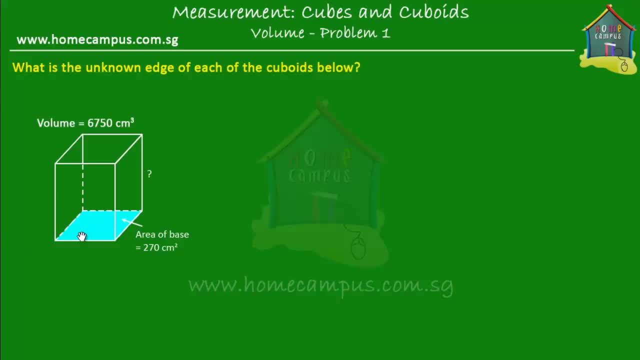 Okay, And let's see what we have here. Well, we have the area of the base. Now let's see what is the base made of. Well, in the case of any cuboid, the base is always made of the length and the breadth. 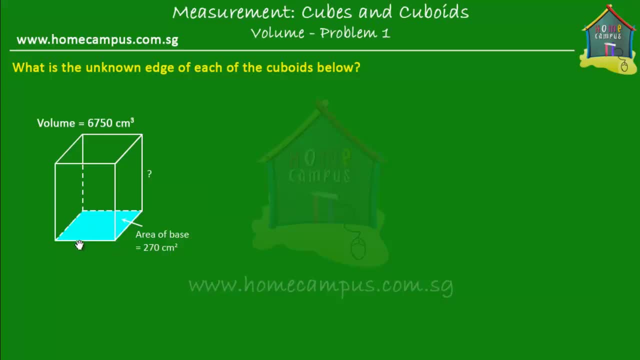 Okay, So here what we know is one of these edges is the length and the other edge is the breadth. Okay, So suppose this is the length over here and this is the breadth of the cuboid, and its area is 270 centimeters square. 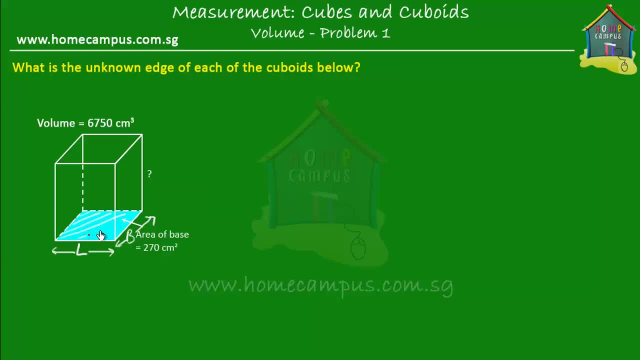 Okay, Now this base Is again a rectangle: All the faces of a cuboid. There are six faces to a cuboid and all the faces are rectangles- either rectangles or squares. Okay, So let's suppose that this is the length and this is the breadth. 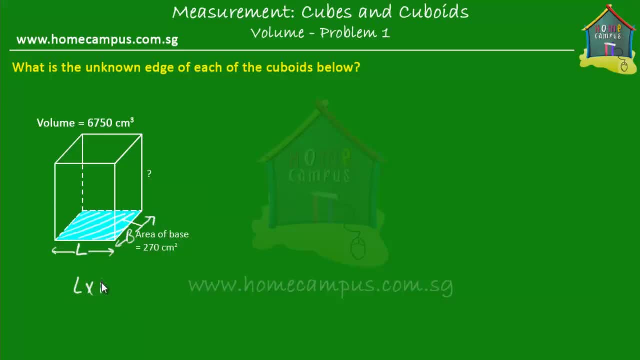 Then the area of this face would be equal to length times breadth right. So the area of this face which is actually the base, the bottom, So the area of the base is equal to the product of the length And the breadth. 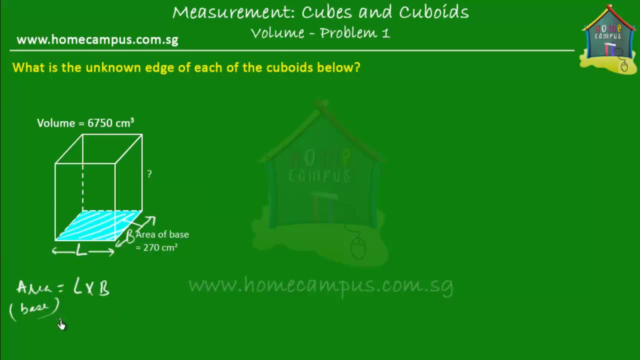 Now, we don't know individually what the length is or the breadth is, but as long as we know that the area is equal to 270 centimeters square, this should be enough for now. Okay, Now again, we plug in what we know into our formula. 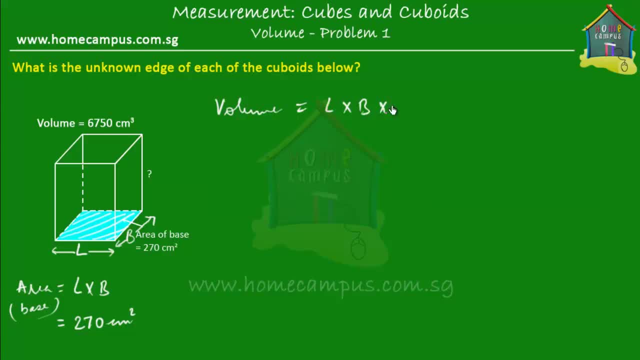 Volume is equal to length times breadth times height. I'm using the short for length, which is L, the short for breadth, which is V, and the short for height, which is H. Okay, Now, length times breadth. We saw just now that 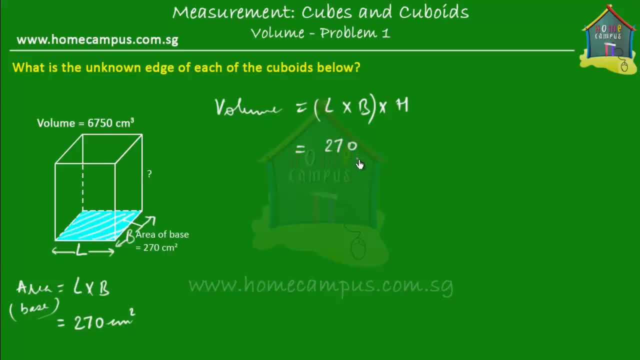 It is equal to the area of the base And in this case this is 270 centimeters square. The height? Well, the height is unknown, So we put H here and the volume is 6,750 centimeter cubes. That's given to us. 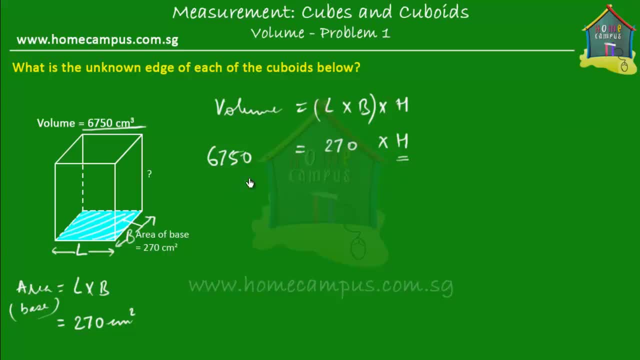 Okay, Now how do you find out what the height is equal to? Quite simply, all you do is you move this number, which is 270, to the other side of the equal sign. So now, what we'll do is: 6,750 will be divided by. 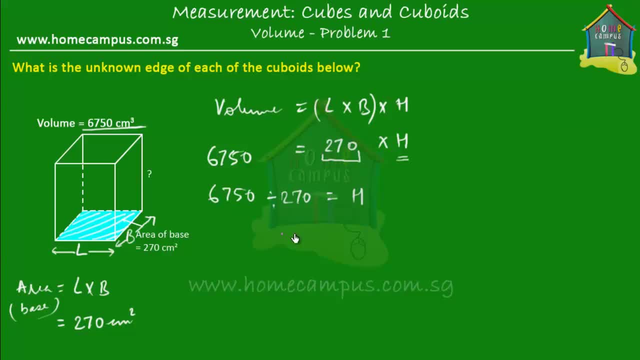 270 to give you the height. Okay, So the height is equal to 6,750 divided by 270, or 6,750 over 270.. I like to do it this way because it makes reducing the number very easy. Okay. 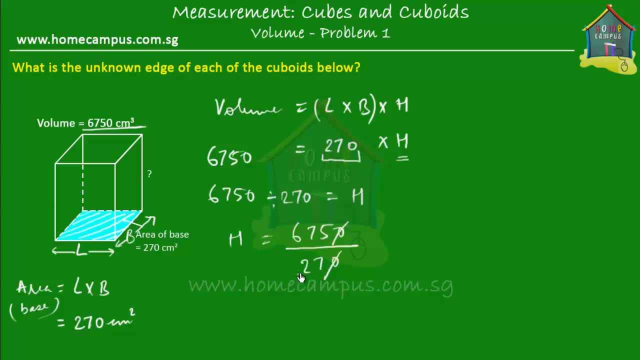 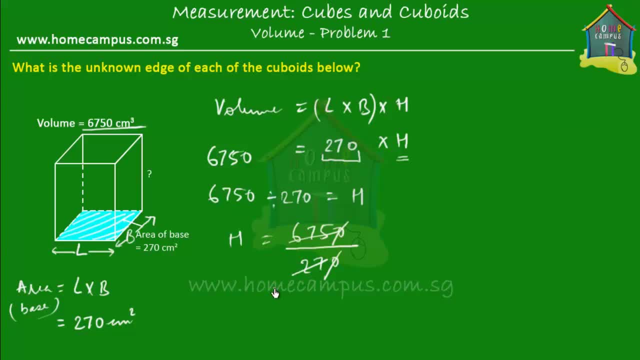 Okay, Okay, Okay, Okay. Keep dividing by small numbers till you cannot divide anymore. Let's divide by three, because we know that 27 can be divided by three, to give you nine and 675.. Well, let's see, Six divided by three is two. 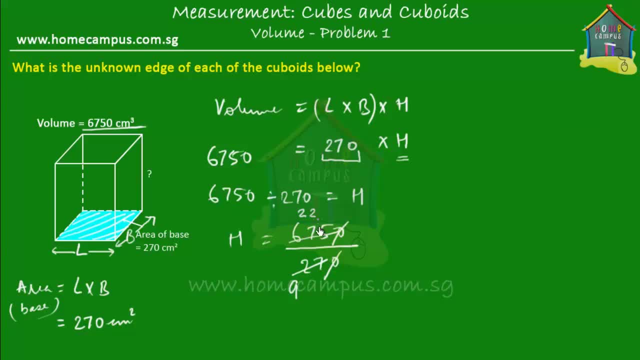 Then no remainder. Seven divided by three is again two, with a remainder of one. So you have 15 here. 15 divided by three is five. Okay, Can we divide that again by three? Let's see: Nine divided by three gives you: 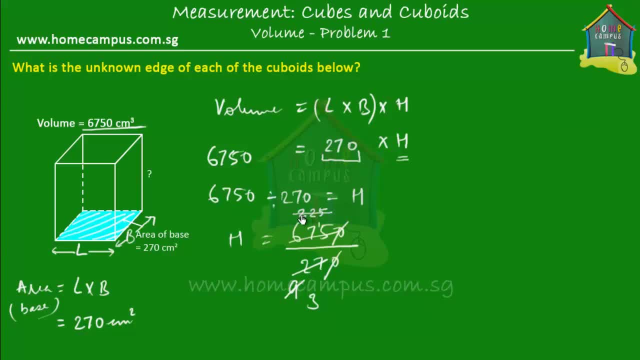 225 divided by three, or 21 divided by three, is seven. You have a remainder of one. So 15 divided by three is five, and this, I know, can be divided by three once more to give you 25.. So here you go. 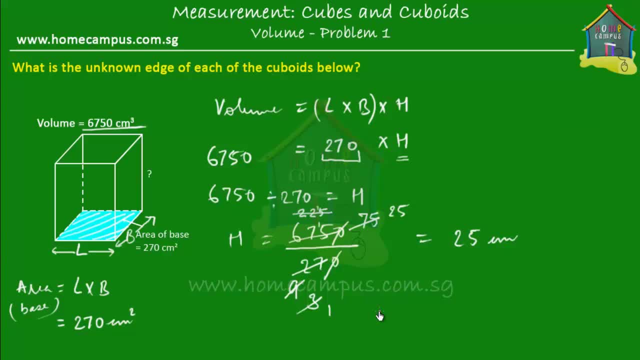 The height is equal to 25 centimeters. That's it. So the unknown edge over here is the height, and that's equal to 25 centimeters. So you see, if you have the volume given to you, okay, and you have to find out one of the edges of the cuboid. 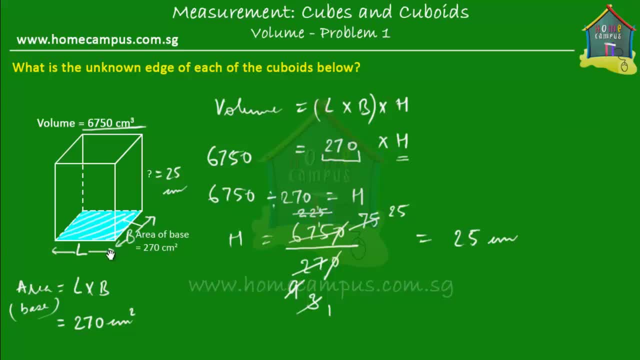 then it's okay if you don't know what the other two edges are equal to, as long as you know what their product is equal to. Okay. So in this case, you know what the base area of the cuboid is equal to, And from that you can find out what the height is equal to. if you also know what the volume is equal to. 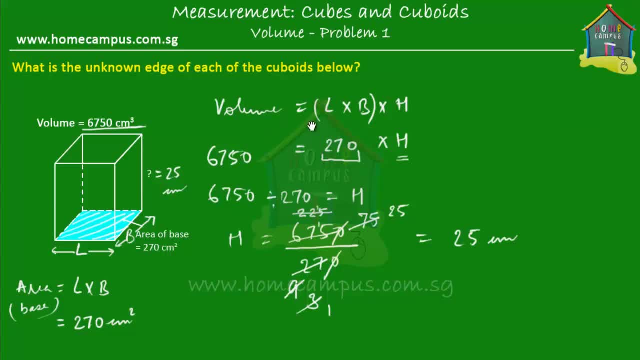 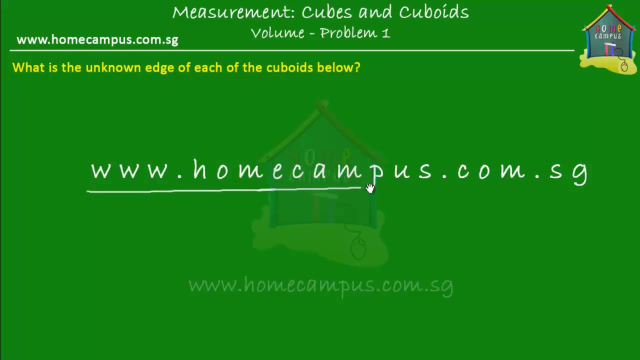 All you have to really remember is the formula to calculate volume of a cuboid, which is equal to the product of its three, Three edges. Well, that's it for now. I hope you understood this lesson and I hope that now you'll go and do some practice as usual at wwwhomecampuscomsg. 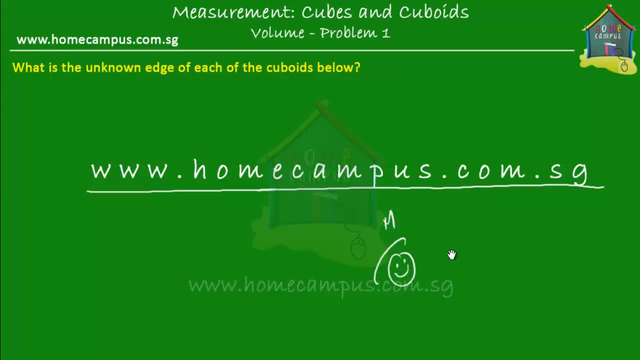 Don't forget to practice, because practice makes perfect. Bye, bye.